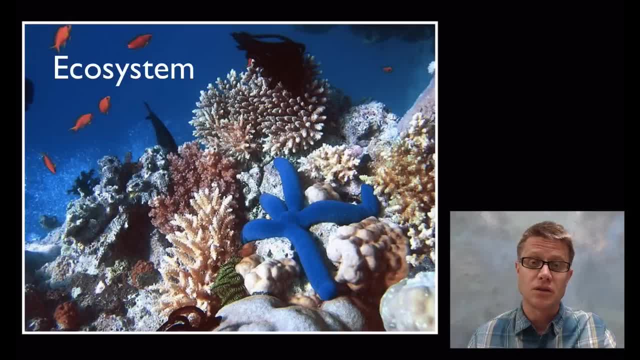 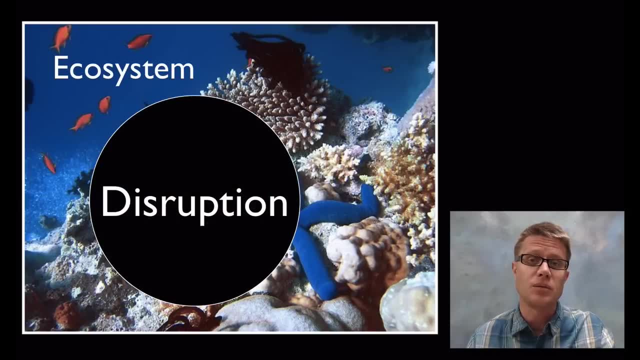 of the nonliving materials. So it's like the water, the temperature, the chemistry, And so if you take an ecosystem like a coral reef and we disrupt it, So we add a disruption, So that could be a change in the temperature or the chemistry, or introducing a new organism. 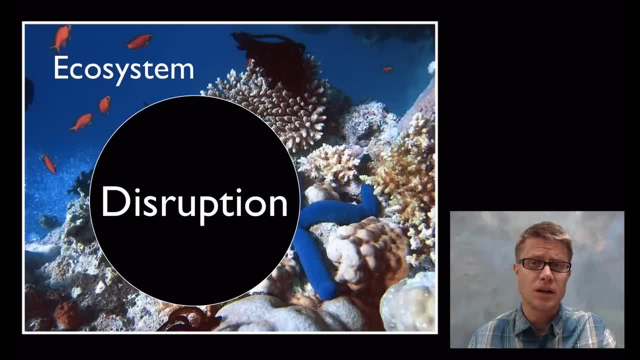 What you're going to do is you're going to change that ecosystem And, as a result, you might see a change in the organism type. You could see different organism numbers. You could have a reduction or maybe an increase. You could see extinction of species. You could. 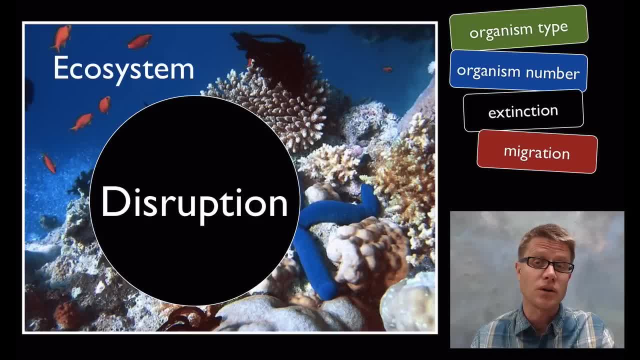 see migration, You could see new organisms coming into the area or organisms leaving, And you could also even see speciation, So the formation of new species And so just disruptions are going to stress an ecosystem And, depending on the health of the ecosystem, 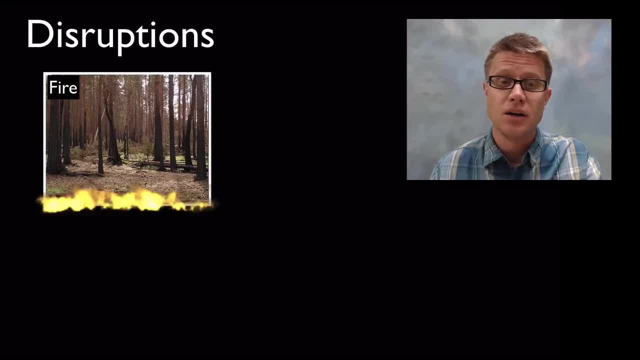 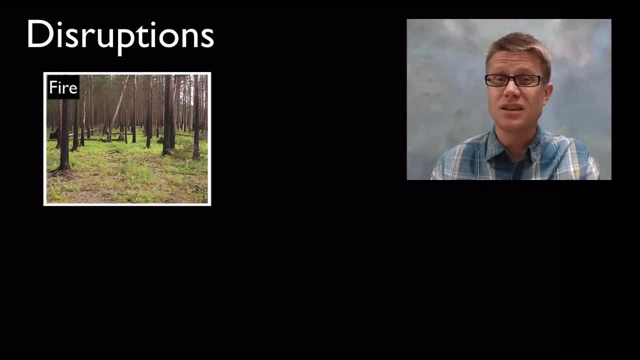 it's going to respond, And so here's some examples: It could be a fire, A fire is going to go through sweeps through a forest, And then life is going to come back after that, But it might not be exactly the same as the life that was there before, Or we could have. 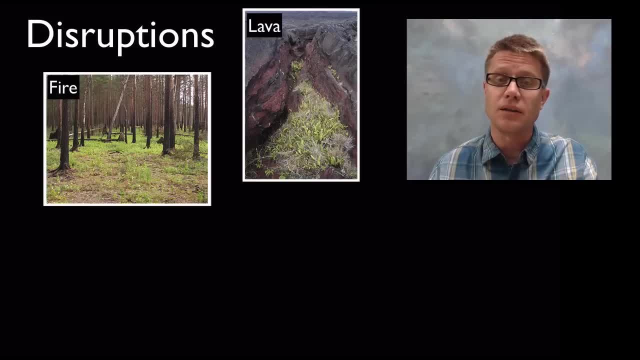 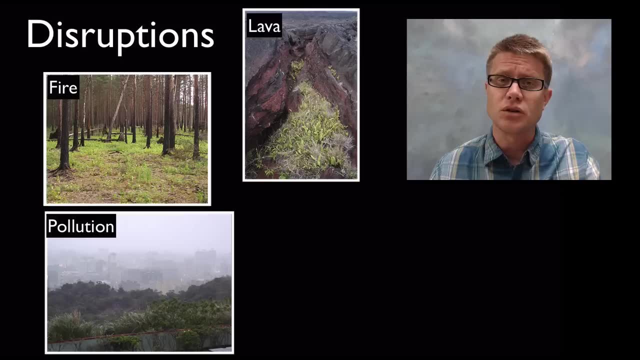 a new rock being formed, So like a lava flow, And then life has to reestablish itself, And so these would be more natural disruptions. Lots of times, humans are causing the disruptions, And so pollution is going to force some organisms to die and some organisms to survive. You, 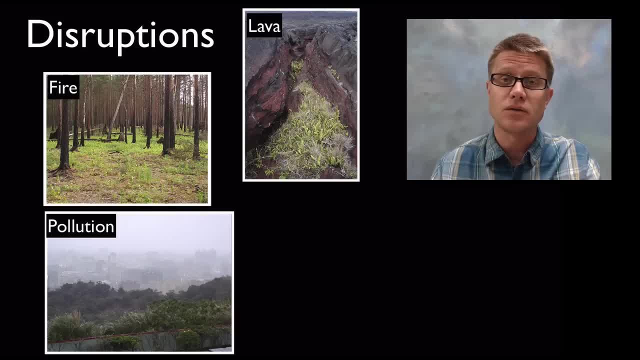 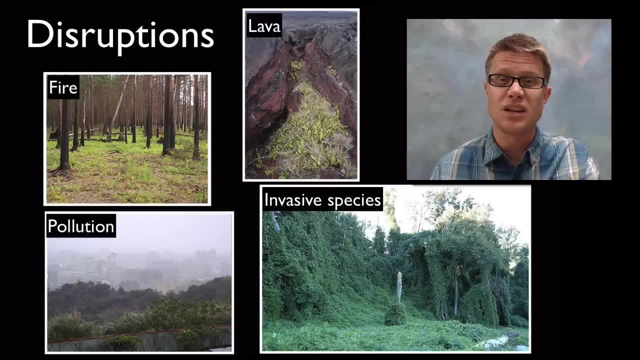 might have new organisms come into an area as a result just of something that we're doing, Or maybe an invasive species. So we brought a plant here, a Japanese plant called kudzu. It didn't have a natural predator And it just spread across the south And, as a result, 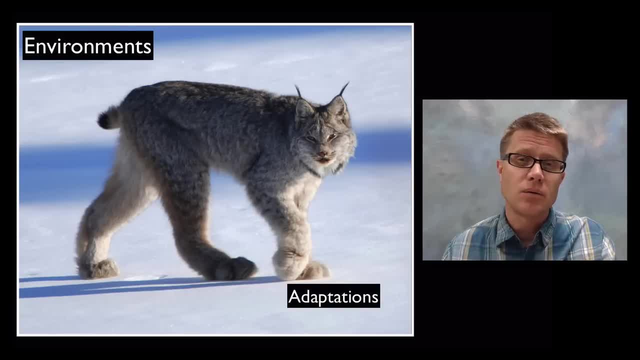 it's changing ecosystems wherever it goes, And so organisms are relatively adaptable. It's adapted to their environment, But everything is constantly changing. So let me give you an example of that. This is a lynx. A lynx is going to be in the northern forest, And 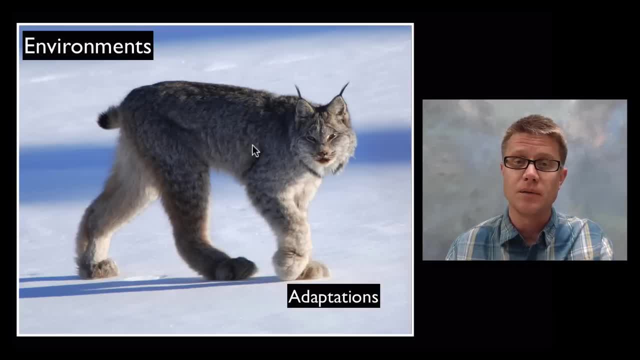 it's evolved to live in a cold kind of a climate. It has these really big feet, It's got quite a bit of fur, In other words, it has all of these adaptations, so it can do well. The reason it has such big feet is so it can run on top of the snow, And so what's going to happen? 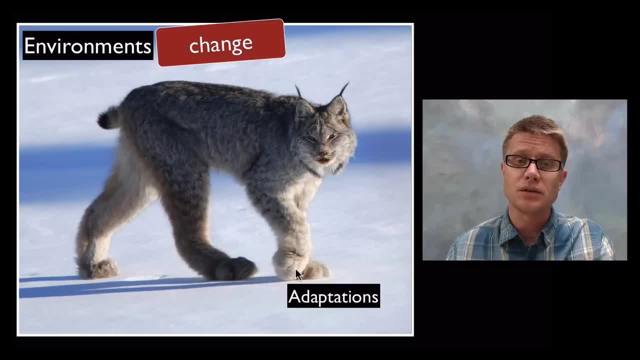 to that environment over the next few days? Well, it's going to have to adapt. It's going to change over the next few decades? Well, it's going to change As we see increases in the temperature, as we see global increases in the temperature that environment is going. 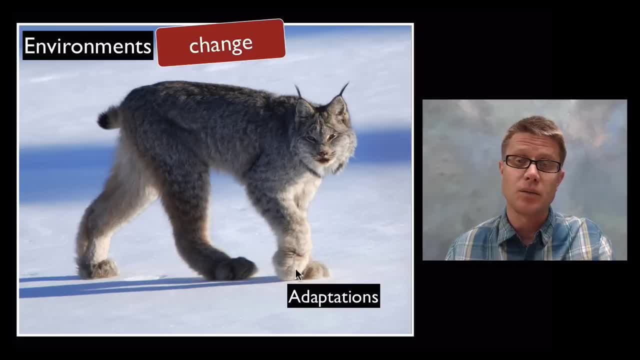 to change. What's going to happen? to lynx with big feet, Well, it might not be as much of an advantage, And so some of them may die, And maybe some of the ones who have smaller feet might do a little bit better, And so that's really what's going on. But the health 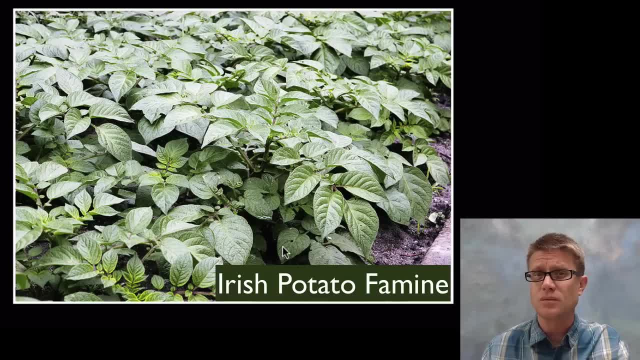 of an environment is determined based on the number of organisms and the diversity of organisms that you have, And so this is a human example, a historical example. So in Ireland, about 30% of the people who were living in Ireland in the 1800s were feeding almost entirely on potatoes. Their 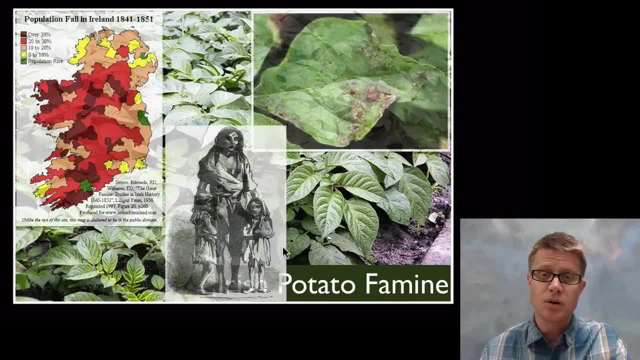 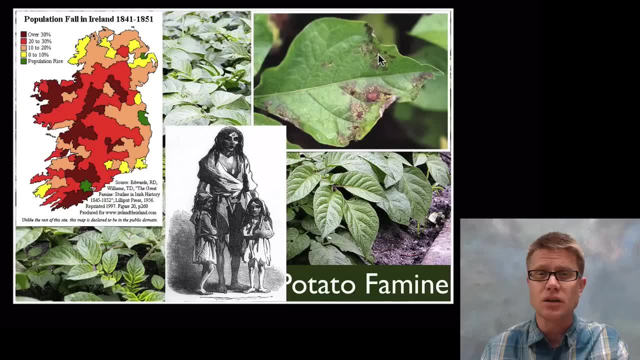 whole diet was based on potatoes, And what happened was the potato famine. So we had a potato blight, And this happened all across Europe, But it especially targeted people in Ireland who were just feeding only on potatoes. So we had this blight, And so what happened? 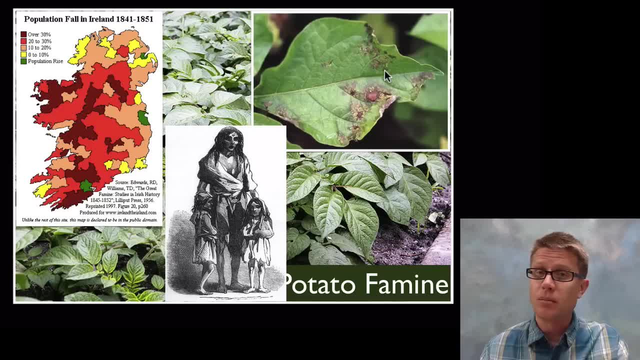 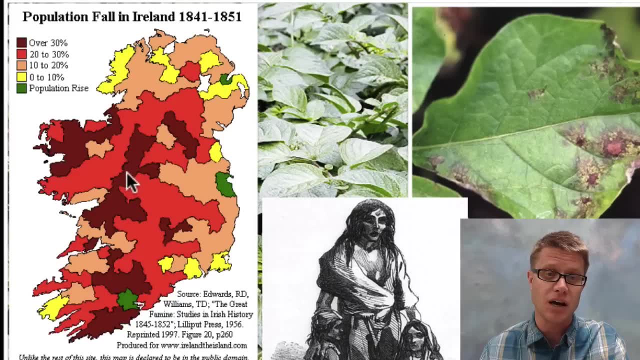 is so many people died. A million people died of starvation and disease in Ireland. A million of them left. And so if you look at this map over here on the side, each of these dark regions in Ireland shows a decrease in over 30% of the population. And so what? 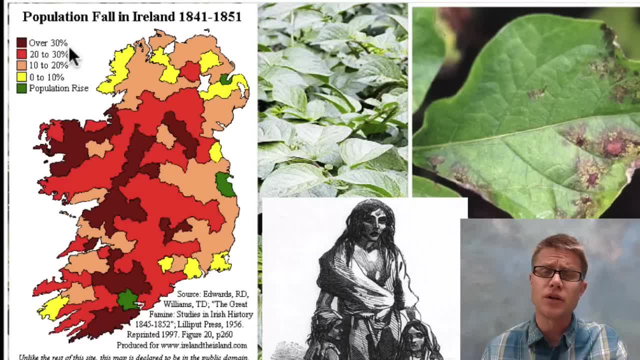 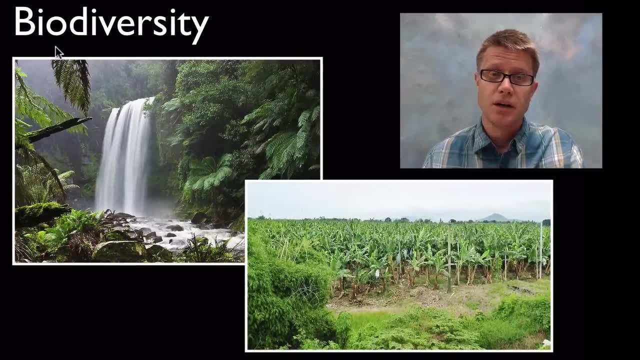 was the problem? The major problem is that they had put all of their eggs in one basket. They were just feeding on potatoes, And so when the environment changed, they weren't able to respond. And so, in Ireland, what happened? Well, this is what happened: The population. 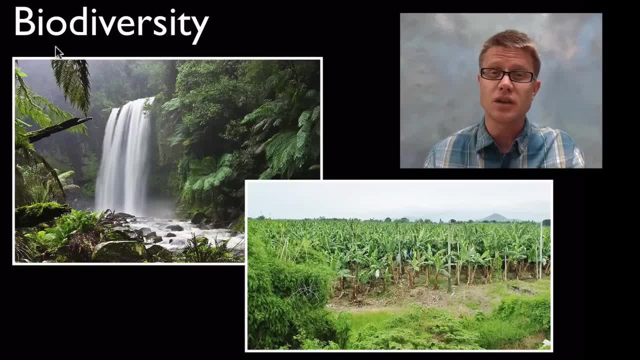 In science we tend to call that biodiversity. Biodiversity is going to be the sum total of different individuals you have in an area, And so if we're looking at a rain forest like this, I can see so many species already, And if we compare that to a plantation here we 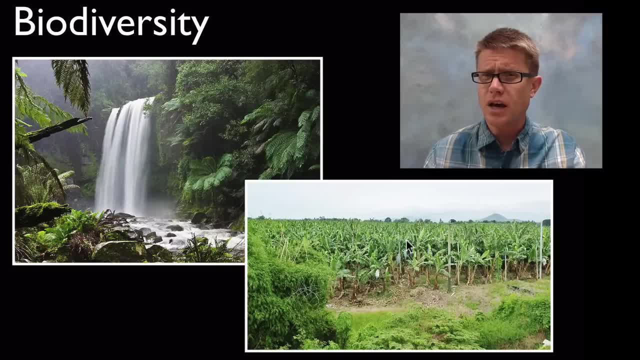 really only see one species out here. And so which is healthier? Well, the one that's more biodiverse is going to be healthier, And what we mean by healthy is that it's able to respond to disruptions or changes in its environment. And so what's the teaching progression? 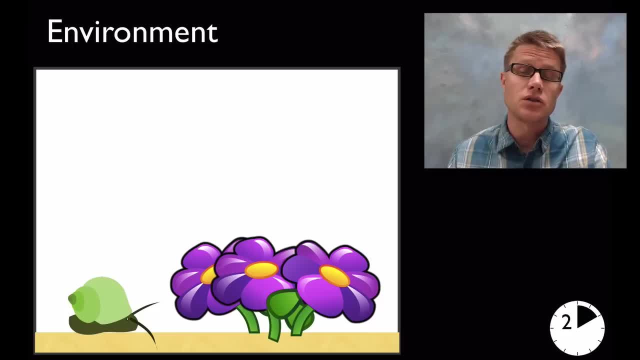 for this. Well, in the lower elementary grades you need to tell your students that plants and animals require things from their environment And if their environment changes, let's say it gets too hot or too cold- that can damage or even kill plants and animals in an area. 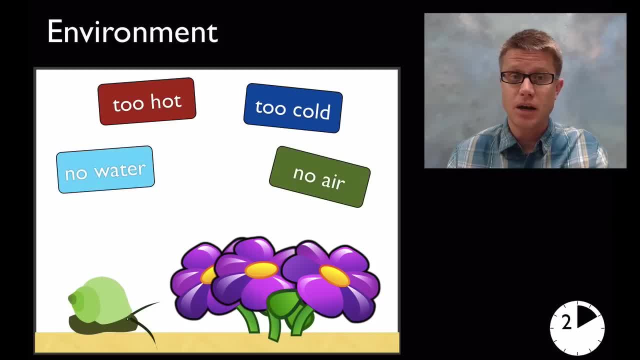 If there's no water, if there's not enough nutrients that they might get from the air, if there's no food in that area, they're going to be damaged and they might even die as a result of changes in their environment. To get more specific, in the upper elementary: 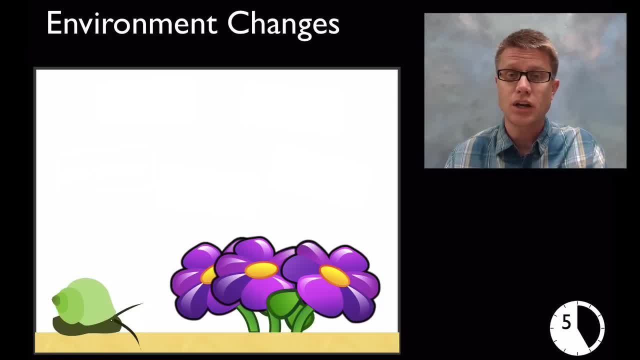 grades. you want to talk about what happens when the environment changes, And so, as we change the environment- no food, too cold, too warm- one thing that could happen is certain species could do well, They could survive and they could pass their genes on to the. 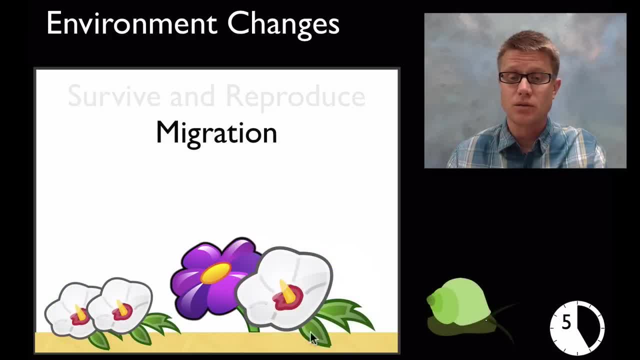 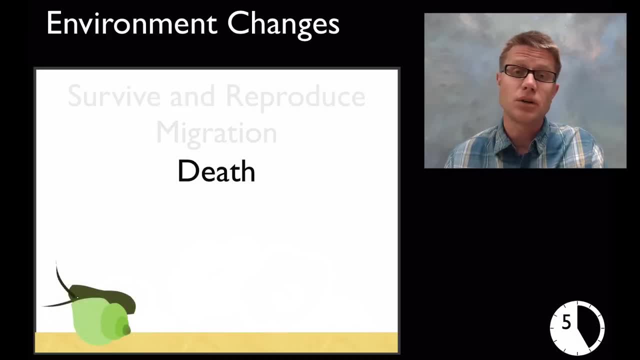 next generation, But they also might migrate. In other words, some species might leave that area and then new species might come in, So we could have migration And then finally we could have death, And so there could be a selective pressure where maybe they don't. 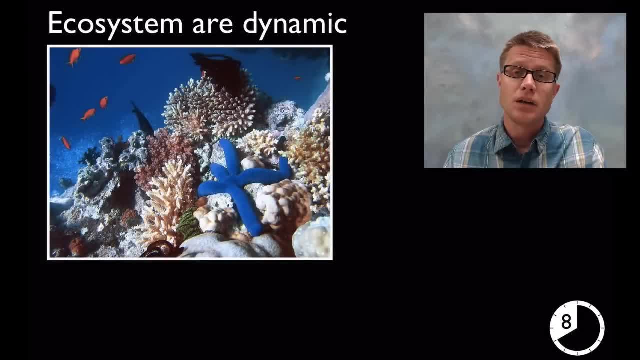 do well as a result of environmental changes. As we move into the middle school, we want to talk about ecosystems. What are all the parts of an ecosystem? And then remind our students that they're incredibly dynamic. They constantly are changing When you look. 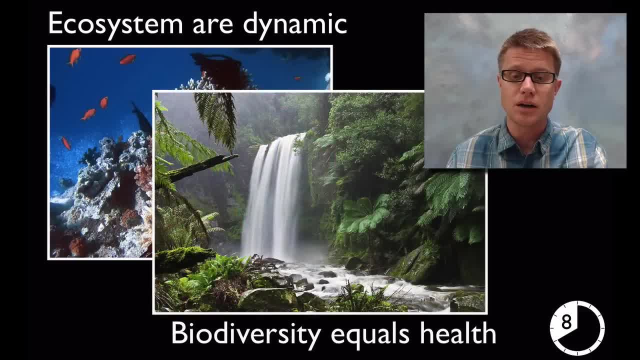 at it, you're just looking at it at one point in time, But they change over time And then remind them that the biodiversity is a good signal of how healthy that environment is, And the reason why is that you have more species And so, as the environment changes, you're more. 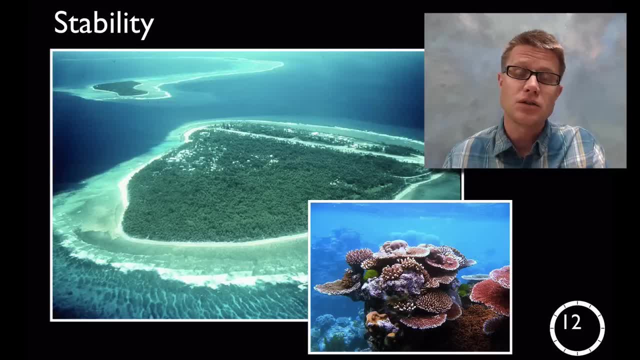 likely to be able to respond to that. And then, finally, as you move on to high school, you want to talk about the stability of an environment, The stability of an ecosystem, And so there are always going to be changes. So if we're looking at a coral reef like this, 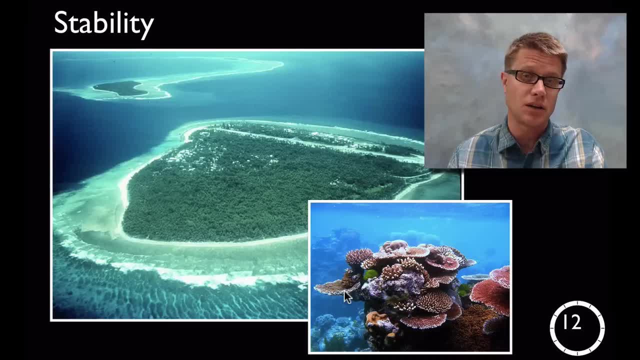 there have always been fluctuations in temperature, Fluctuations in chemistry, Small changes and small fluctuations of organisms coming in and out, And they remain stable over time. But sometimes it changes too quickly and they can't do well. So right now we're seeing huge